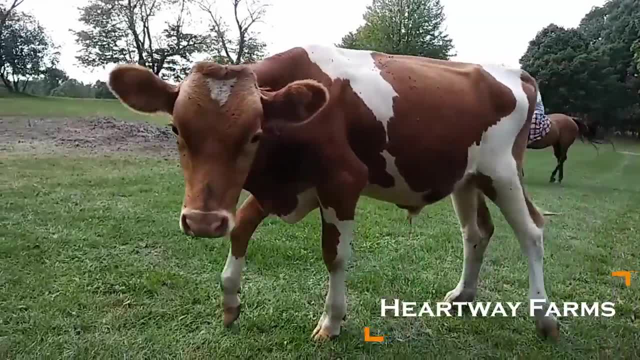 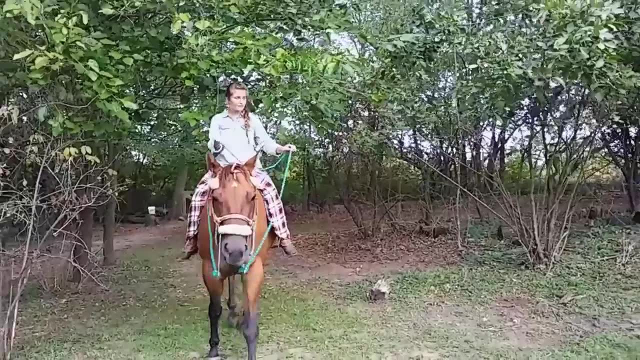 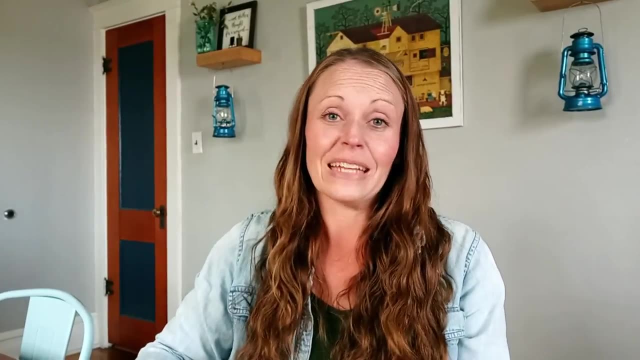 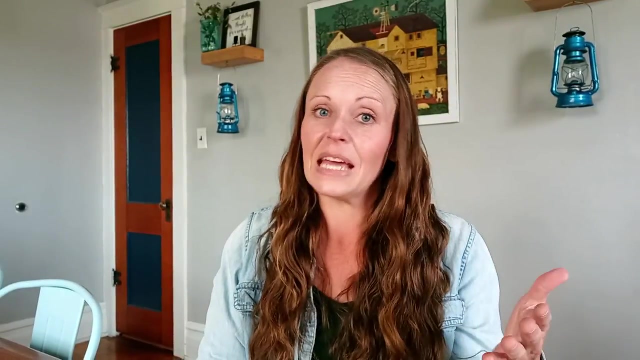 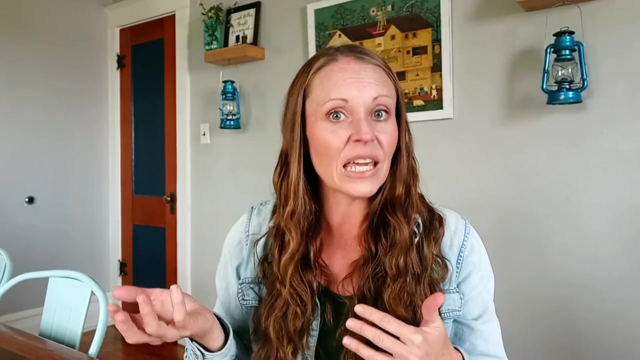 We all know that when you have children, things change, But one of the things that changed for me when Julianne was born was that I began to investigate and research a lot of the items that we had in our home, And then I was deciding if they were worth keeping or to be thrown in the 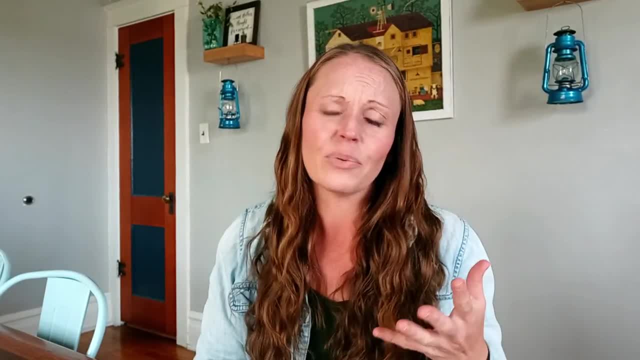 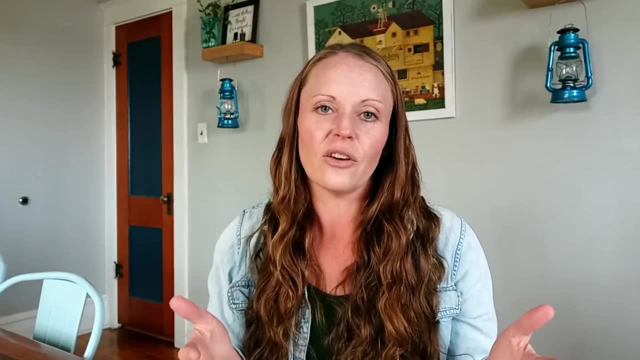 trash, And so I began to research all of the bath and body products that we were using, as well as the food we were eating. all of these things, And it can be a little bit overwhelming, but that was the beginning of my all-natural journey, trying to find things that were good for our bodies. 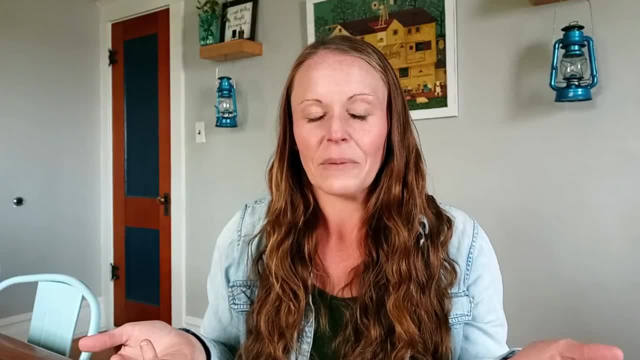 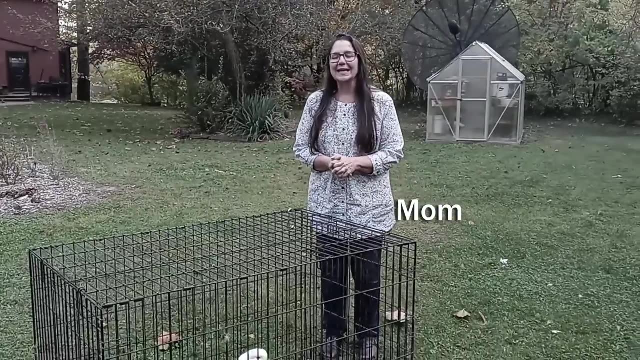 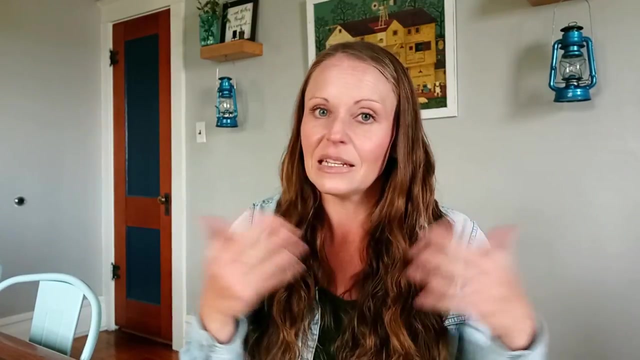 inside and out and wouldn't harm my family. Well, back in 2009,, a few years after Julianne was born, my mom began doing the same research as well And she started making her own soap, And she has blessed my family and my siblings and many family members with these products that she 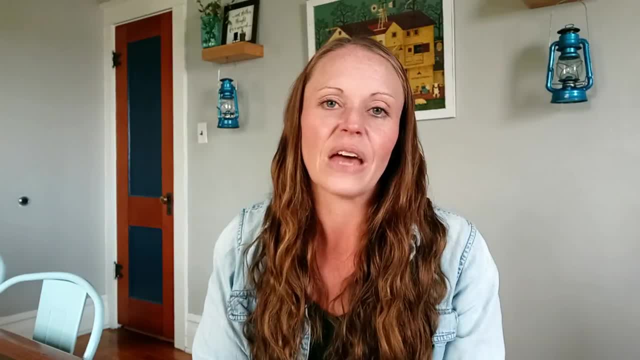 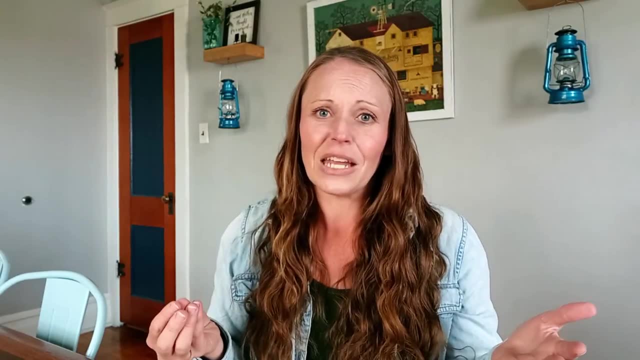 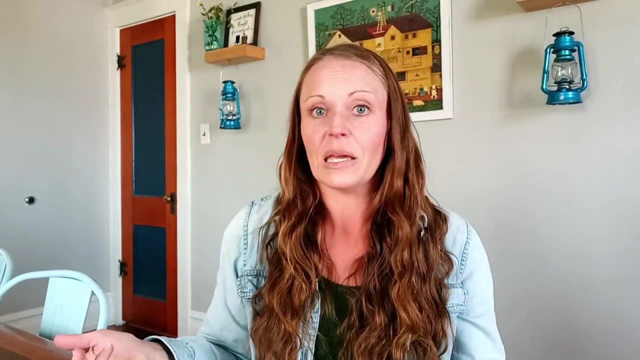 makes soap and lip balm and lotions and all of that that are made with good, clean ingredients and will not harm our bodies. So we've been able to take advantage of that for many years. Well, in recent years here, Julianne has shown an interest in taking over the soap making business. 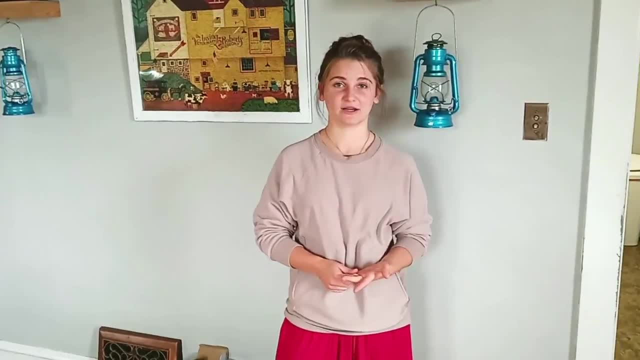 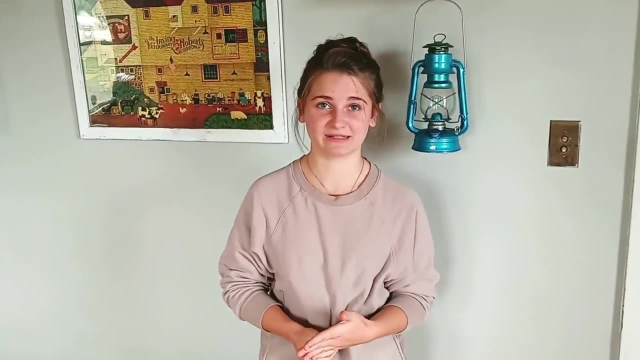 as well as making lotion and lip balm. So a couple of months ago I approached my grandma asking her if she would teach me to make soap, And now I've taken over the Heartway Farm soap business pretty much 100% of the time. I really enjoyed learning how to make soap and doing it. It's really fun. 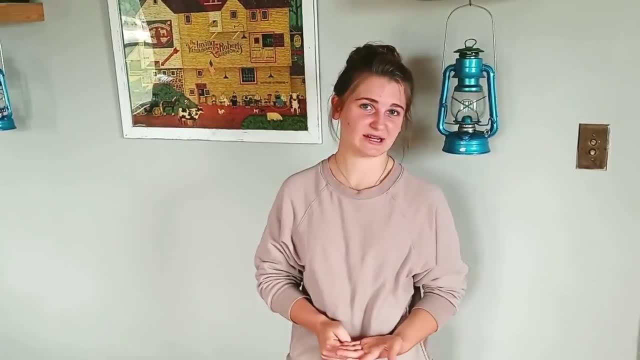 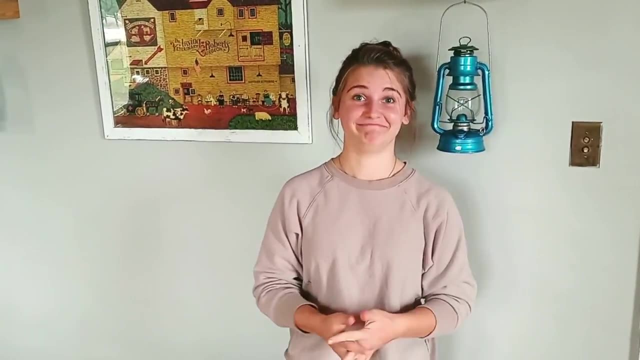 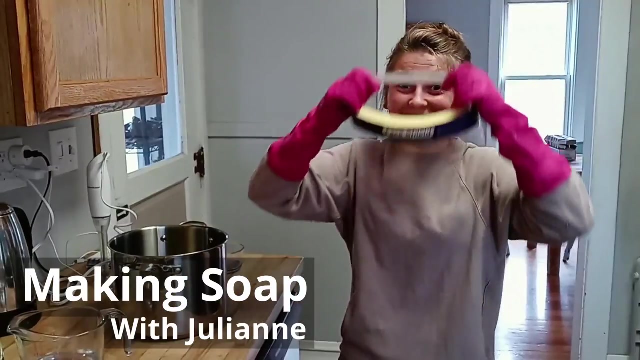 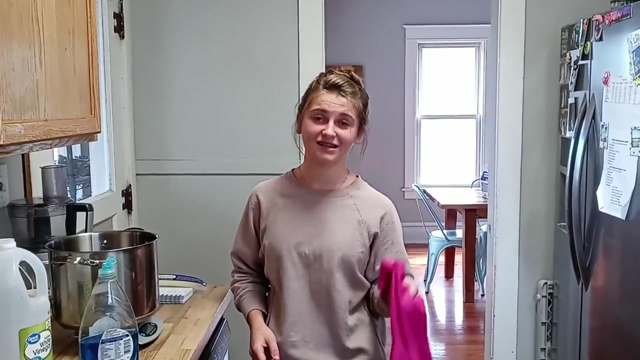 but you also do need to use quite a bit of wisdom when doing it, just because it can potentially be dangerous if done improperly. So today I need to restock my lavender and tea tree soap, so let's make soap. So, because we are going to be working with lye today, there are a few safety. 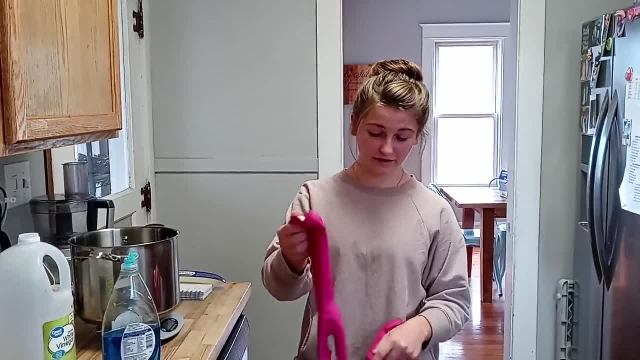 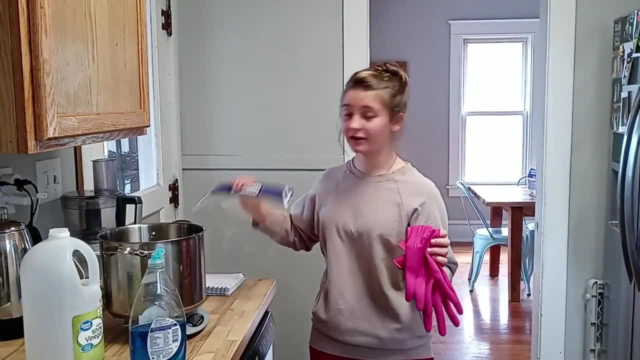 procedures that you pretty much always have to follow. One of those is wearing gloves that come up to your elbows, so lye does not come in contact with their skin. Another one is wearing something to protect your face, whether it's goggles or gloves, And then the other one is wearing a. 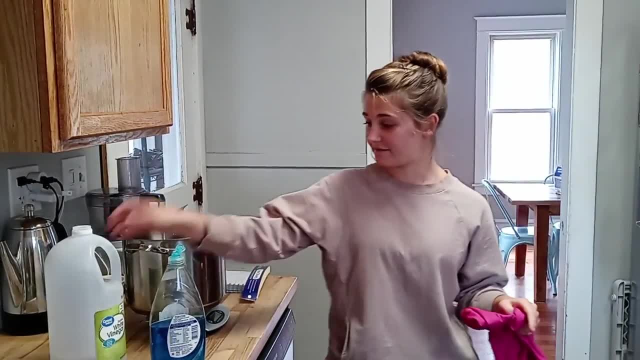 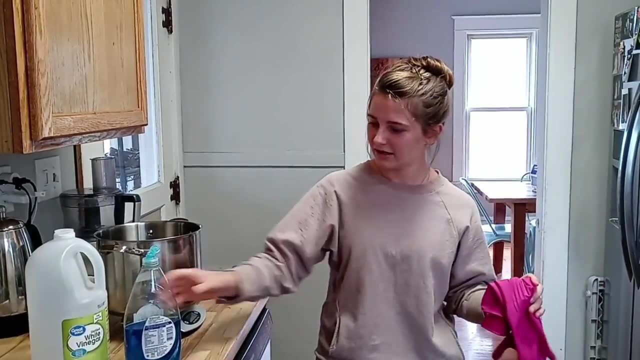 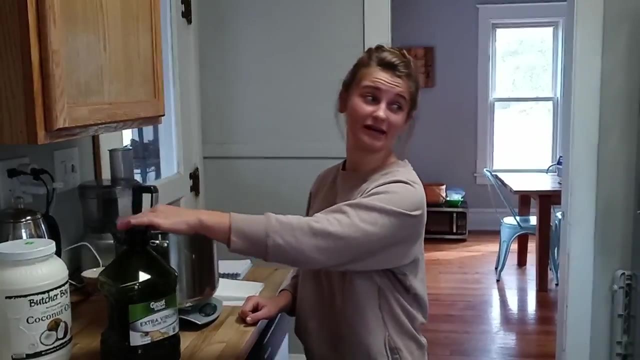 face shield is what I like to use. Another one is having white vinegar on hand, because it neutralizes lye if it gets on your skin or on the countertop or anything else, Degreasing dish soap in case anything needs to be washed. So our first step is you have to weigh and melt down the oils. 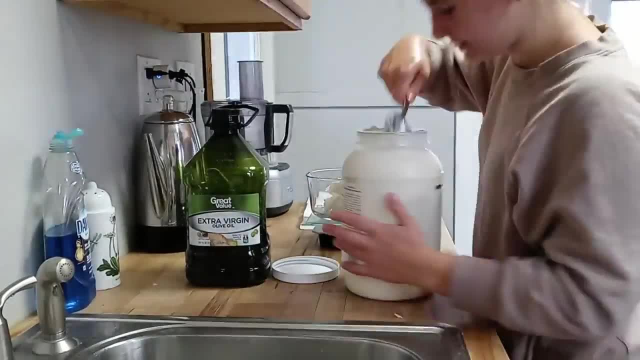 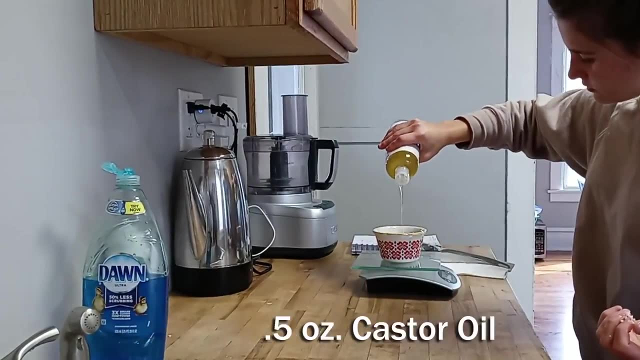 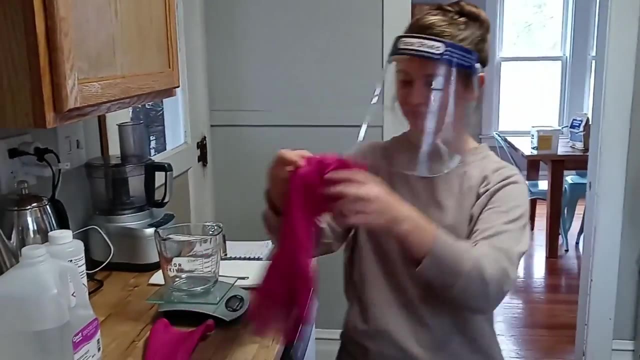 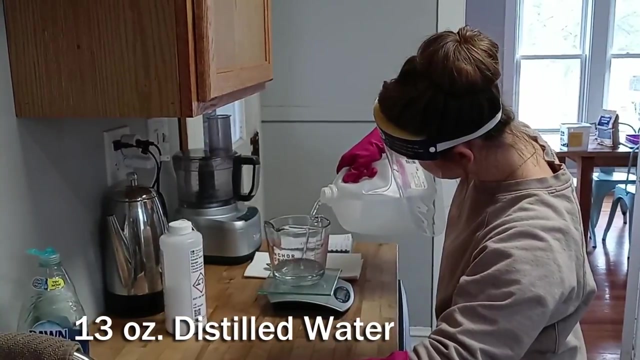 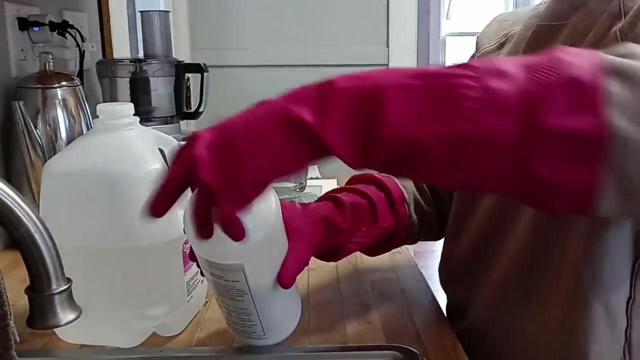 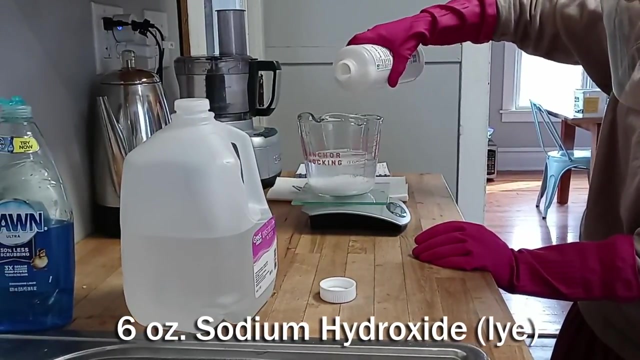 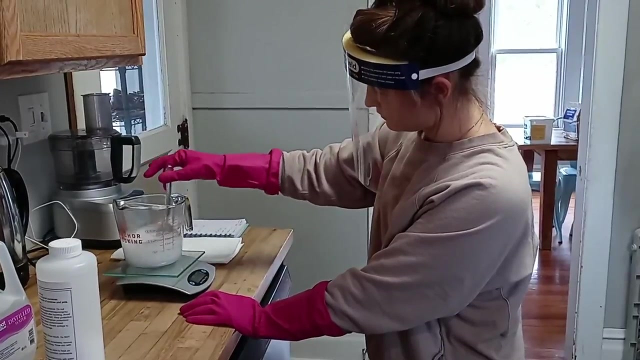 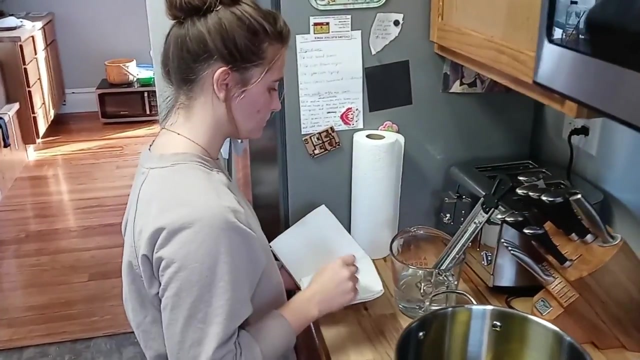 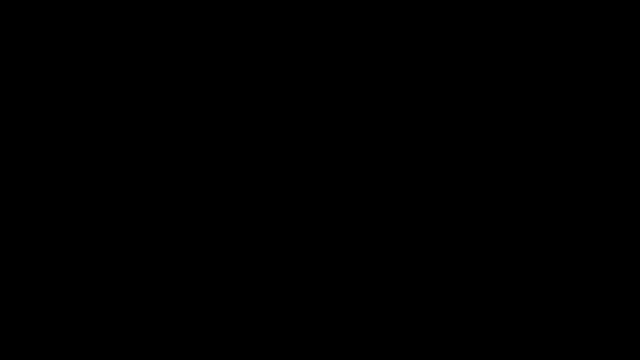 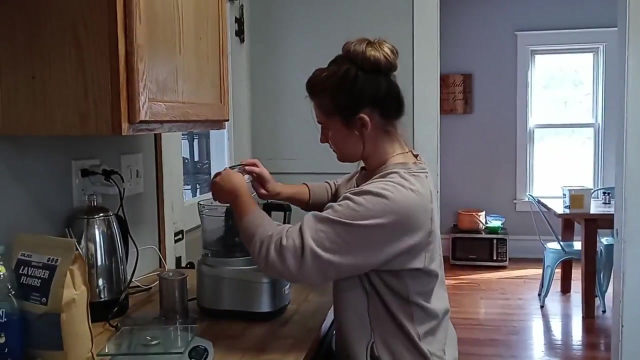 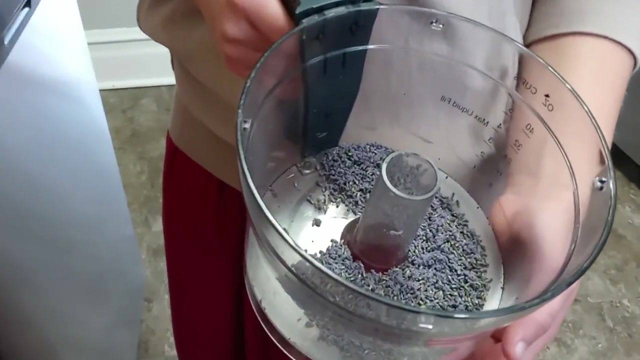 So the second step is we need to measure out our lye solution. So while we are waiting for our lye solution and our oils to come to proper temperature, I'm going to prepare my lavender flowers. So the last step is mixing together our lye solution and our oil solution to make the actual soap. 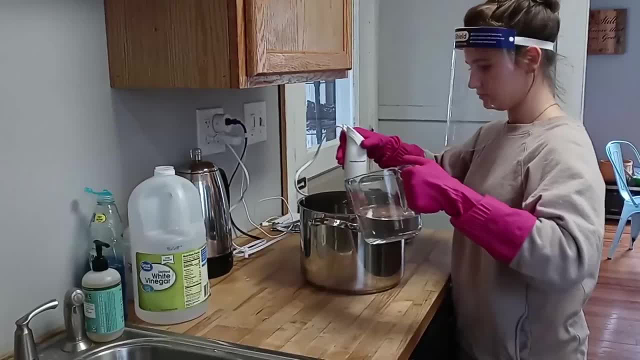 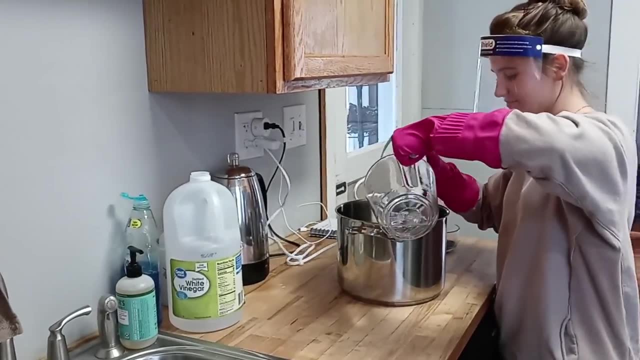 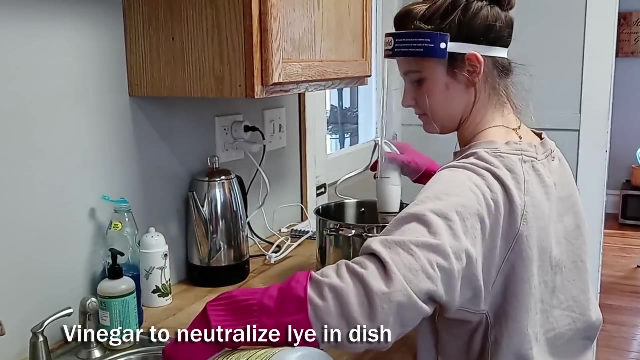 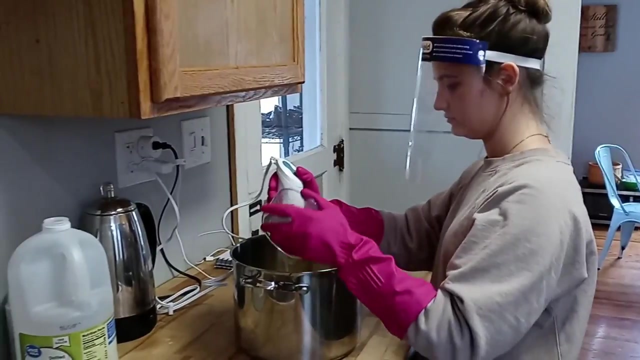 So I'm going to gear back up again. Let's go. Here goes the trashcan with oil on the side. I'm going to separate out the lye solution and put it out on the lye tube. You are strongly forbiden to use those lye soaps. 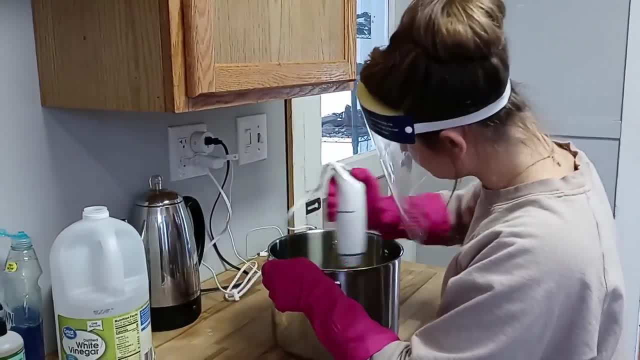 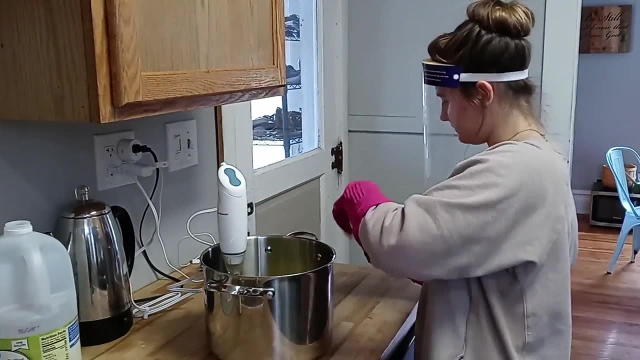 How do they come to a suitable temperature? I'm not going to be using any lye soap, But they can get mixed together. I'm not going to be using any мороз, So I don't have to. went to the lye. 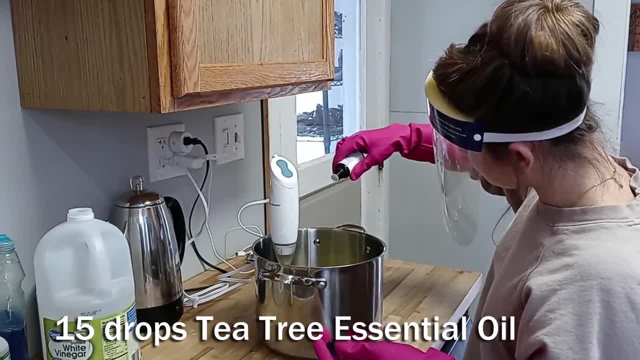 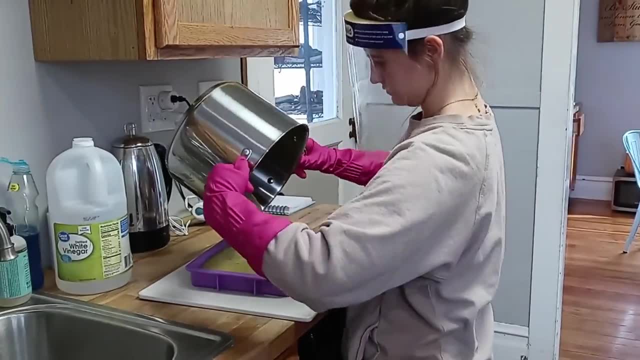 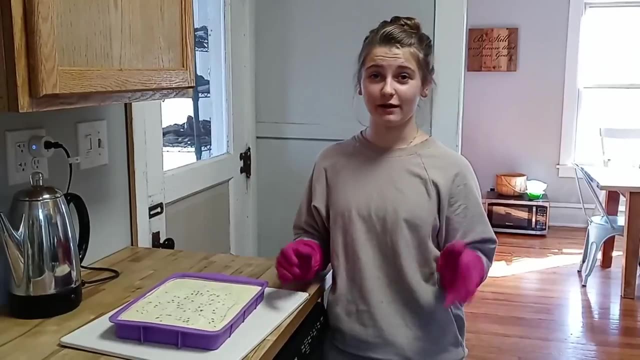 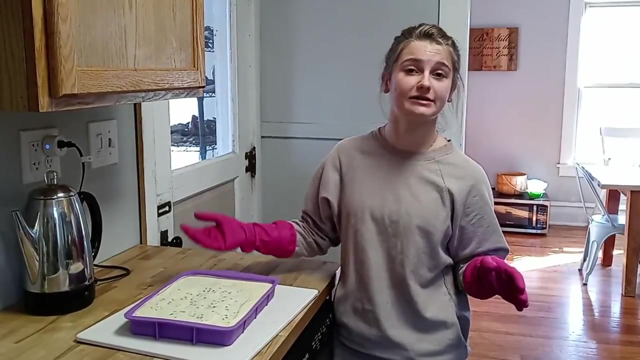 And now it's time for our plants to also come into contact with the soil and make sure. So now I'm going to put this soap in a nice child proof location for two days, and at the end of the two days I'll take it out of its mold and cut it into bar shapes and then put.